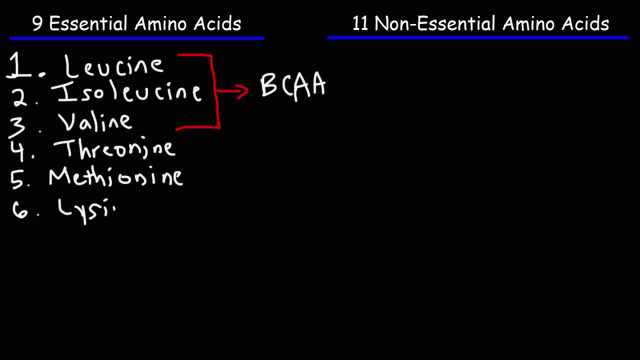 Next we have lysine. Lysine is a precursor to carnitine. Number seven, phenylalanine: It's basically alanine with a phenyl group. Now phenylalanine is a precursor to tyrosine. 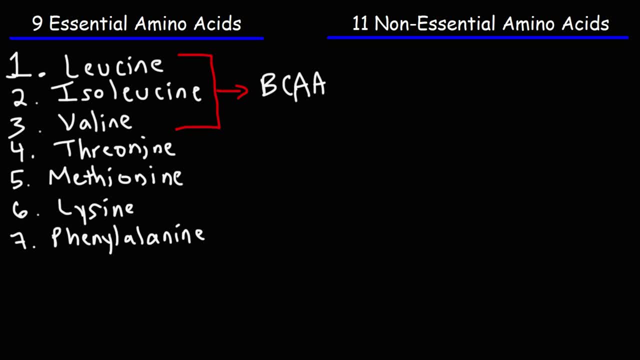 And tyrosine. Lysine is a precursor to neurotransmitters like dopamine, epinephrine and norepinephrine. Number eight, histidine. Now this particular amino acid is a precursor to histamine, uriconic acid and also carnosine. 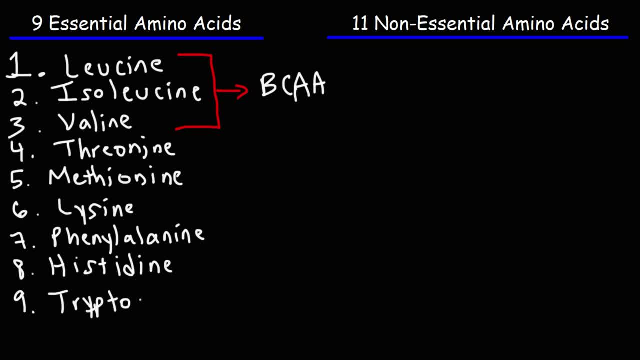 Number nine, tryptophan. So this particular amino acid is a precursor to serotonin, which regulates a person's mood, and melatonin, which is involved in the sleep-wake cycle. So those are the nine essential amino acids. 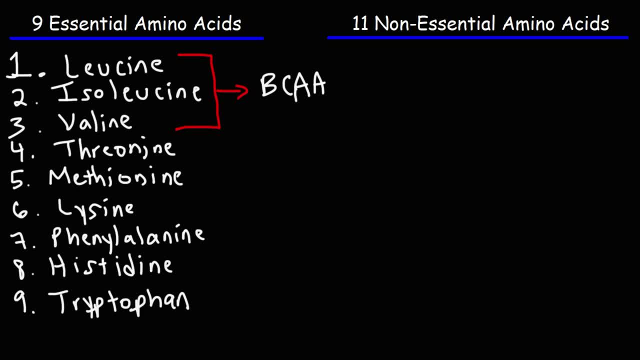 Now, what makes them essential? They're essential due to the fact that your body cannot synthesize these amino acids on its own, which means you have to apply them to your body, Which means you have to obtain it from your diet. The best way to do this is to eat a variety of foods and vegetables. 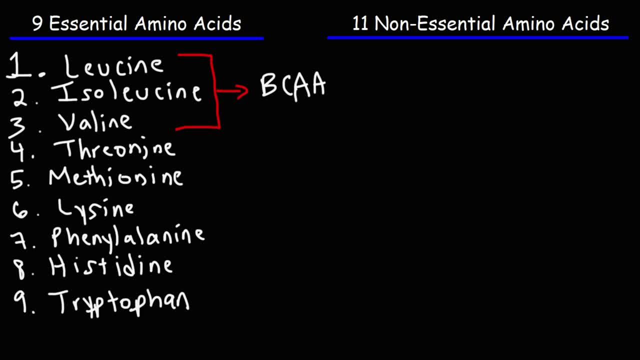 rather than just eating one particular food. Because, let's say, if your diet consists of mainly one food, you might be deficient in one or more of these amino acids. So to avoid deficiency, it's wise to eat a variety of plants, vegetables and other foods. 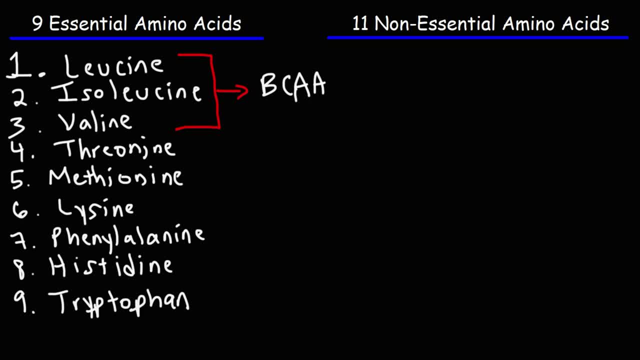 Now let's talk about the 11 non-essential amino acids. Number one: we have cysteine. Next tyrosine. So keep in mind, these amino acids are non-essential because your body can make these amino acids. 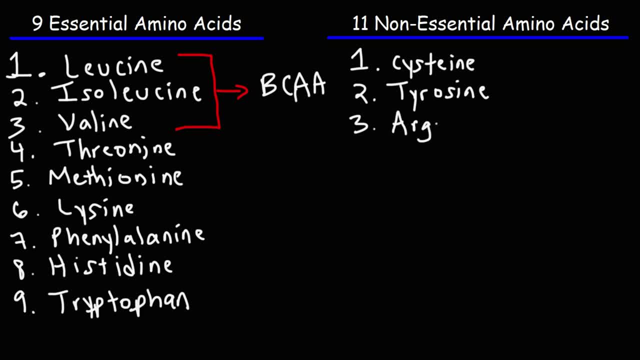 Number three: arginine. Next up, we have aspartic acid. It's also called aspartate in its depronated form. And then you have glutamic acid, also known as glutamate Glutamate, When the carbosilic acid loses its 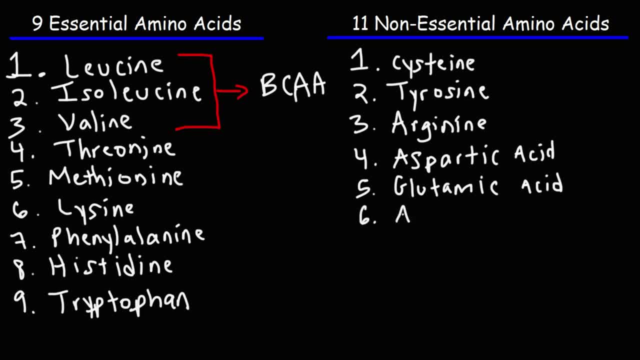 Next we have asparagine. Asparagine is very similar to aspartic acid. Instead of the carbosilic acid functional group, you have an amide instead, And the same is true for glutamine: It's very similar to glutamic acid. 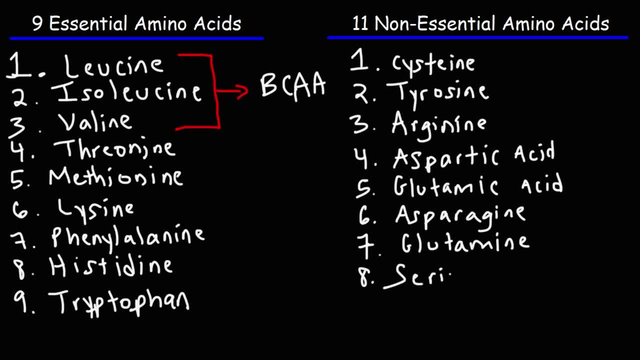 Number eight, serine, Number nine, glycine, And number 10, proline, And the last one is alanine. So those are the standard non-essential amino acids. Now cysteine is considered an amino acid that is conditionally essential. 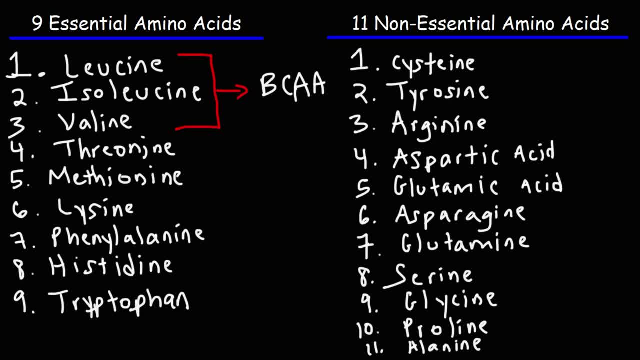 What does that mean? Well, there are some times where you may need to get it in your diet, particularly if you're low on methionine. If your body has enough methionine, it can produce cysteine. Your body can produce cysteine using methionine and also serine. 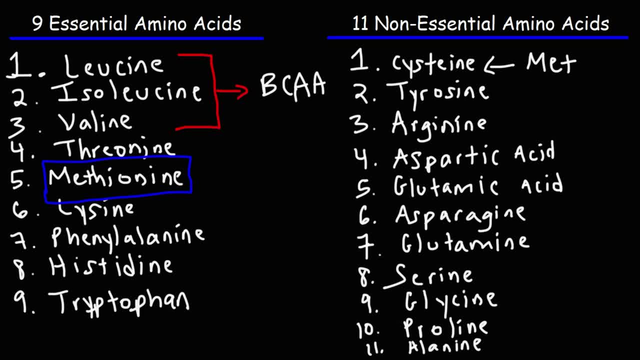 So it is conditionally essential. So if you have enough, If you have enough serine and methionine in your body, then it can make cysteine. Tyrosine is another conditionally essential amino acid because it can be produced from phenylalanine. 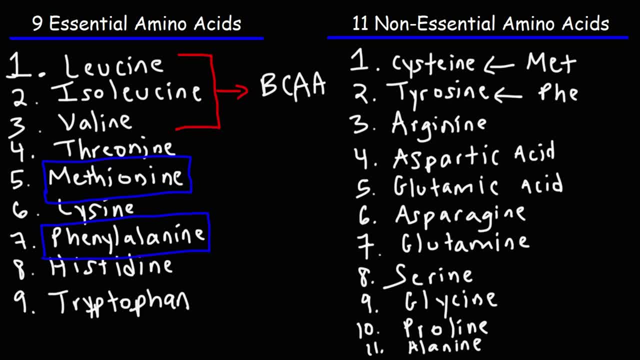 So as long as you have enough phenylalanine in your body, your body can make tyrosine. If you're deficient in this amino acid, then you need to get this in your diet. If not, you're going to be deficient in tyrosine as well. 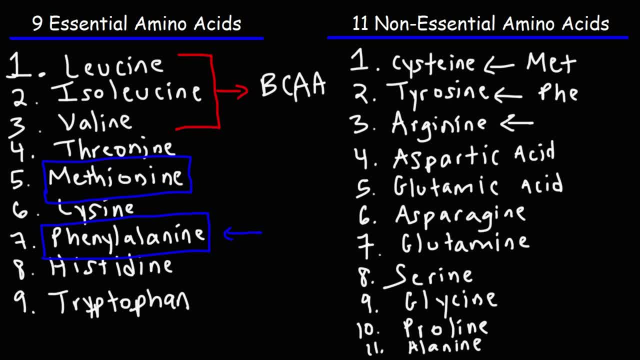 Now, arginine, by definition, is not an essential amino acid because your body can make it. However, it's typically considered conditionally essential because, even though it can be synthesized, it's often needed in greater amounts than the amount that your body can synthesize. 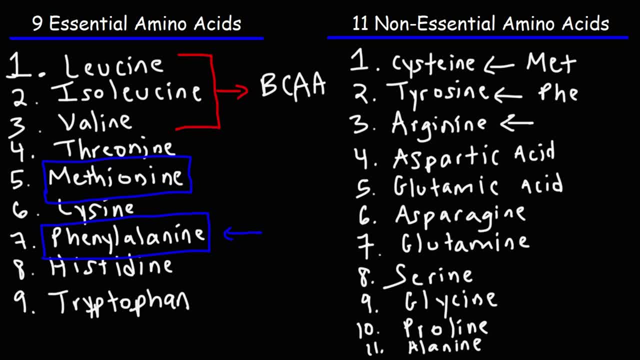 So, basically, the demand is greater than the production with this particular amino acid. So these are three that are conditionally essential. Now there are other amino acids that can be conditionally essential, dependent on certain conditions, Let's say if your body is under stress or if you're fighting illness, or for women, if they're pregnant. 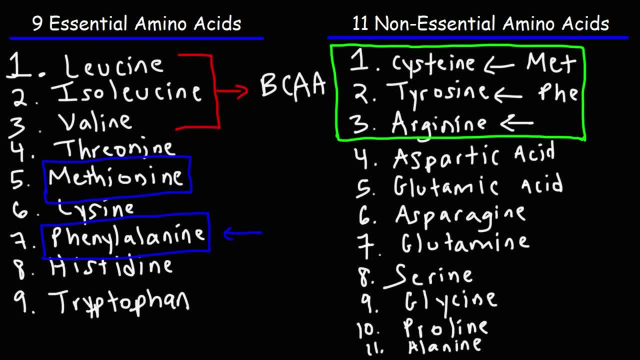 certain amino acids may be consumed more than others, which can make them conditionally essential, But the best way to make sure you get all of your amino acids is to eat a variety of foods, So you can eat a variety of fruits, vegetables and different types of foods. 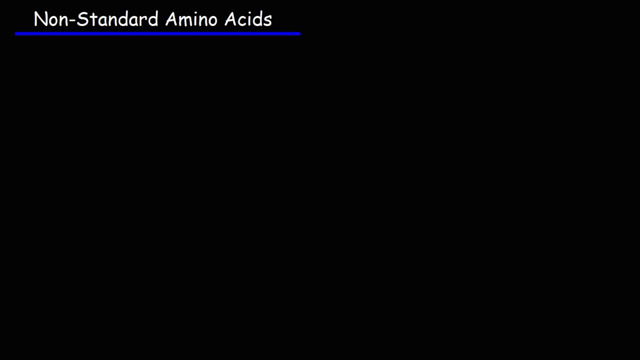 So far we've considered 20 of the standard amino acids, The 9 essential amino acids and the 11 non-essential amino acids. But there are some other amino acids that occur in nature, So one of them is hydroxyproline. 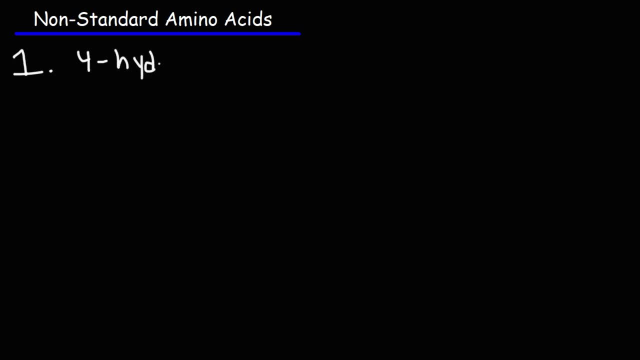 Specifically 4-Hydroxyproline. So this is basically proline with a hydroxy group attached to it. There's also 5-Hydroxylysine. Now these two modified amino acids. they occur naturally in collagen. 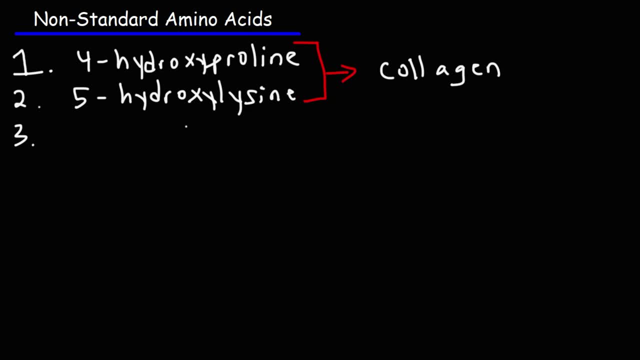 But these are non-standard amino acids. They have a very specific structure. So they're not just an amino acid that is considered to be a proline, They also have a very specific structure. So this is what we call a beta alanine. 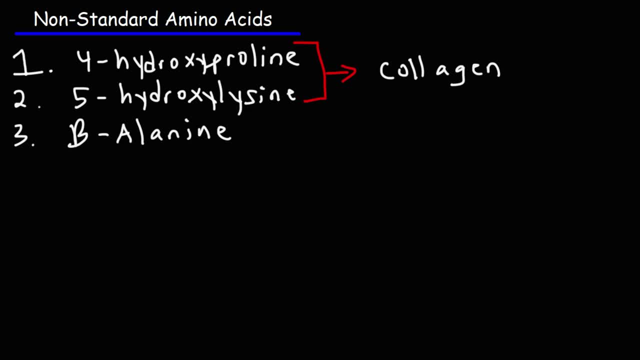 Beta alanine is a limonene precursor to the dipeptide carnosine, which is composed of beta alanine and histidine. So if you don't have a beta alanine precursor, you can use a beta alanine precursor to get a beta alanine precursor. 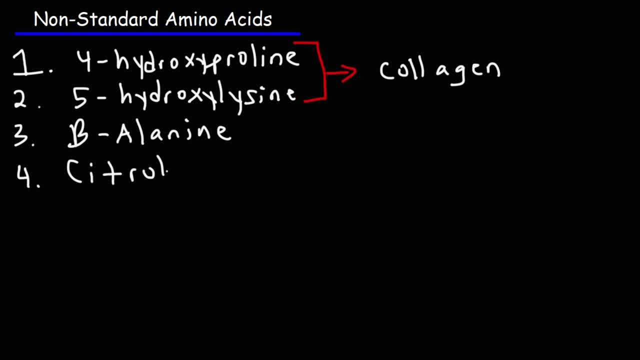 Another non-standard amino acid is citrulline. Citrulline is produced from aromatase, which is an amino acid, So it's a very common amino acid. So that's a very common amino acid- arginine when it is used to produce nitrogen oxide. So citrulline is the